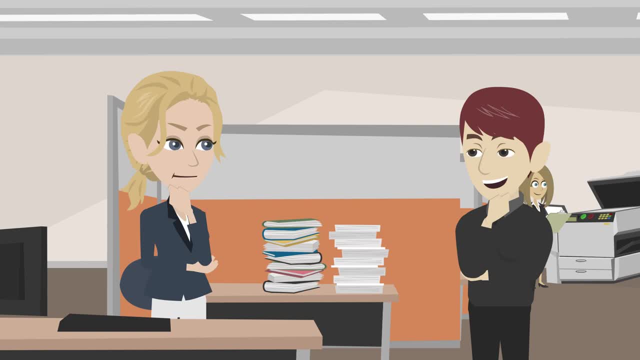 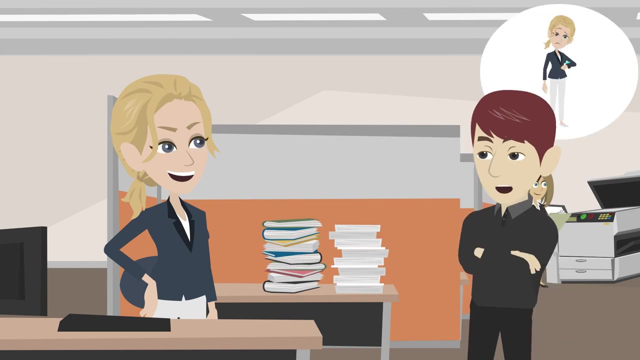 to get used to it and see results. Time will tell if it's a waste of time and money or not. Well, it seems like you're putting a lot of time into it. It just doesn't seem like it's time well spent. 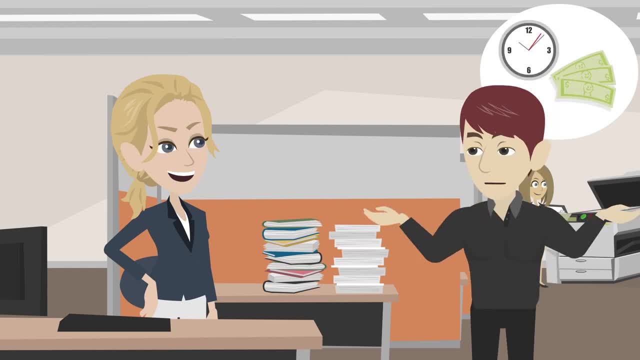 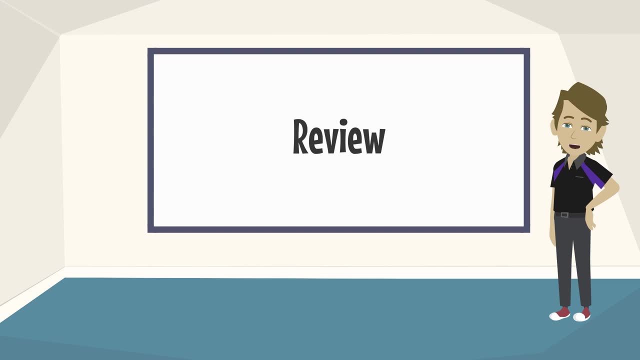 You know time is money, Dorothy. Let's review some of the vocabulary and the expressions of time. First, let's look at oversleep versus sleep-in. Oversleep is something that you do by accident To sleep longer than you intended or planned. 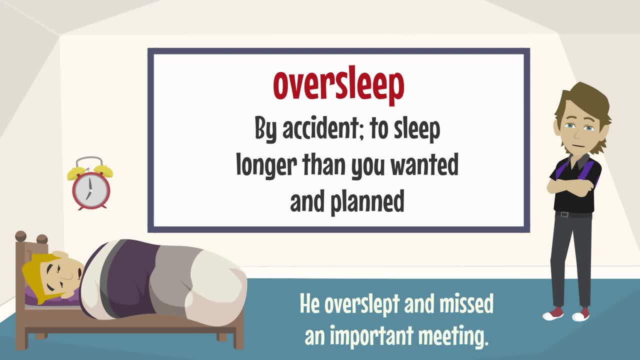 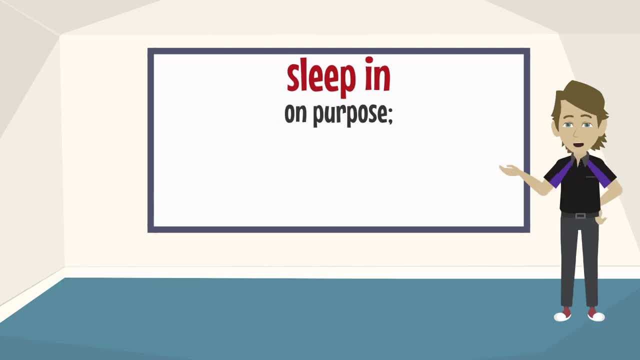 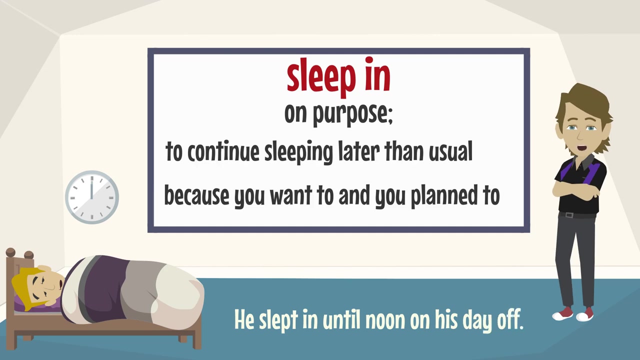 For example, he overslept and missed an important meeting. Sleep-in is something that you do on purpose To continue sleeping later than usual, because you want to and you plan to. For example, he slept in until noon on his day off. 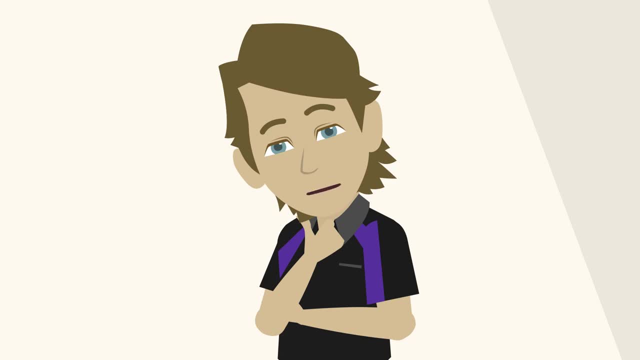 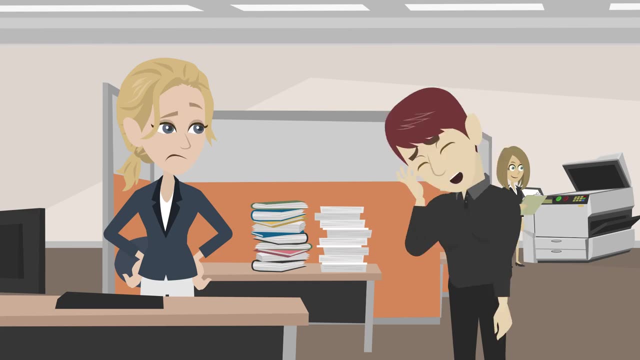 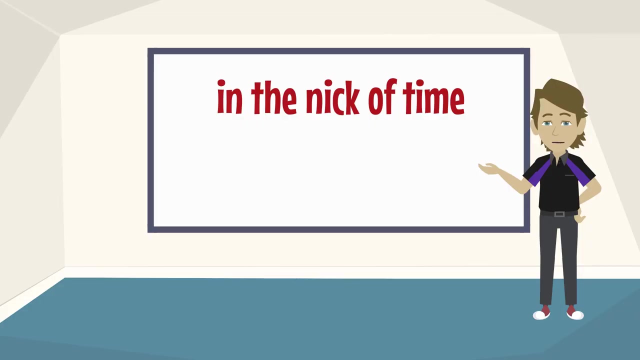 Now let's look at these in context again. Did you oversleep again? Yes, I'm afraid I did. I like to sleep in. The next expression is in the nick of time. We use this expression when something is done just before something bad will happen. 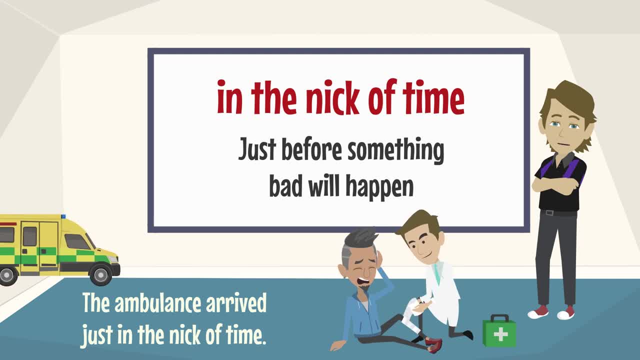 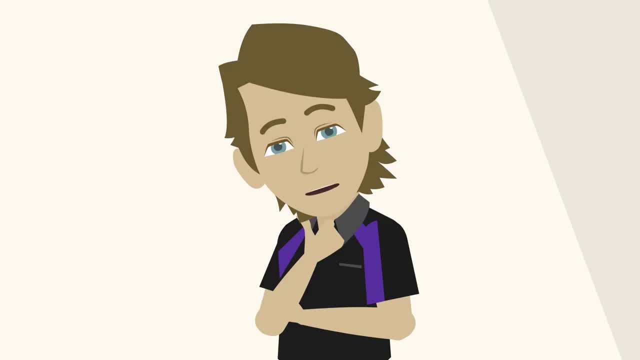 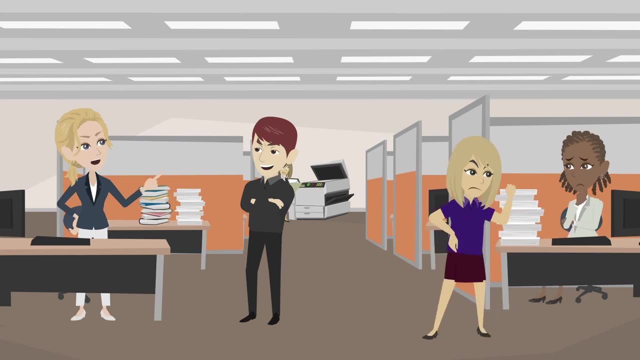 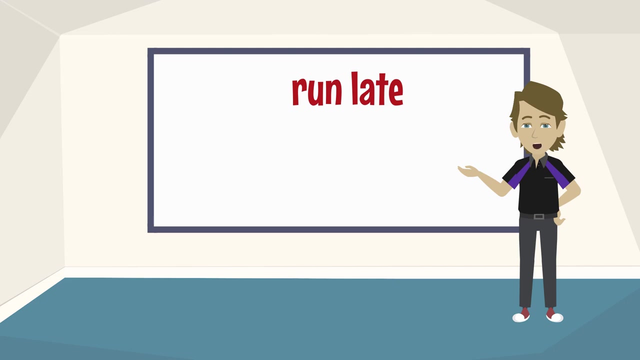 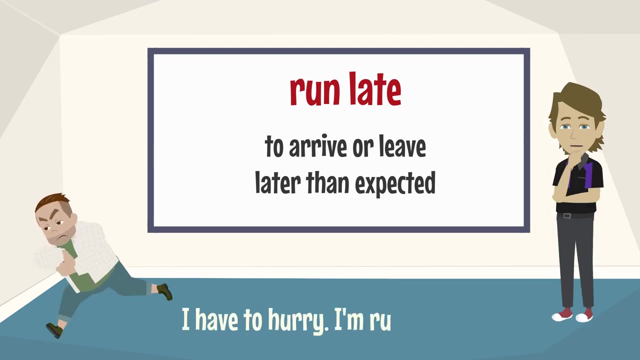 For example, the ambulance arrived just in the nick of time. Let's look at it in context again. Our next expression is run late. Run late is to arrive or leave later than expected. For example, I have to hurry, I'm running late. 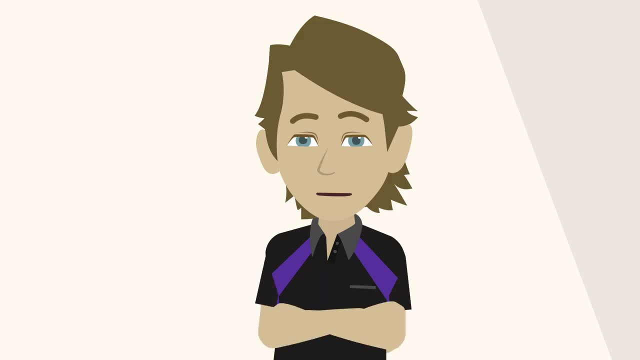 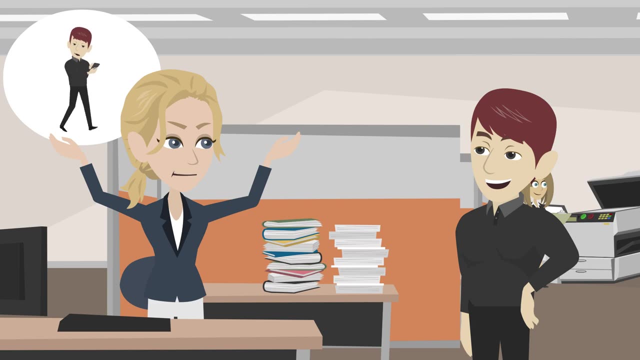 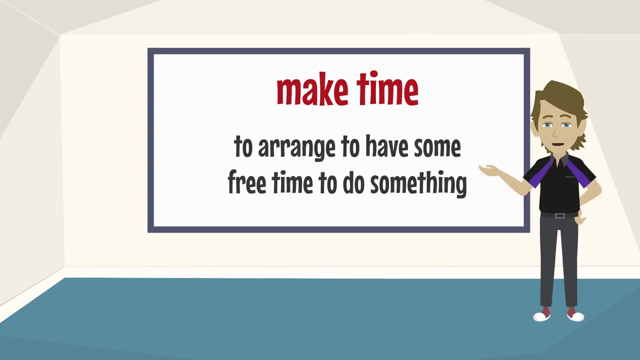 Let's look at this again in context. Next time you're running late, message me and I'll cover for you if Sandy is around. Our next expression is make time. Make time is to arrange to have some free time to do something. The doctor will make some time to explain everything to you. 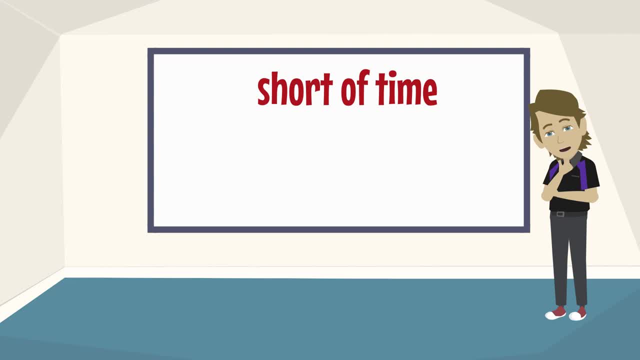 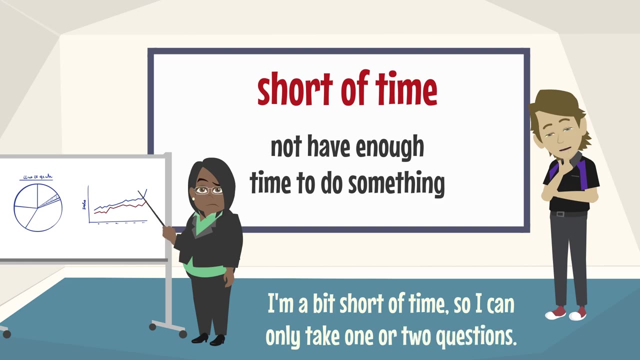 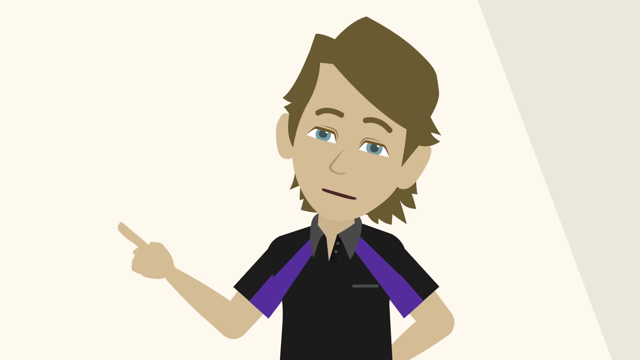 Our next expression: Make time is short of time. To be short of time is to not have enough time to do something. For example, I'm a bit short of time so I can only take one or two questions. Let's look at these expressions in context again. 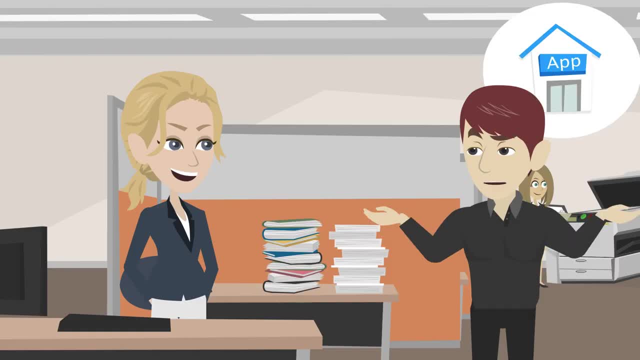 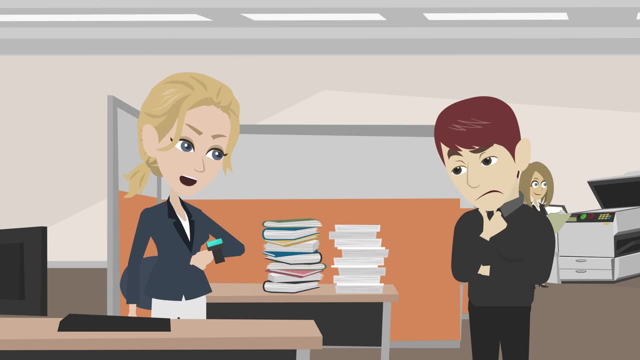 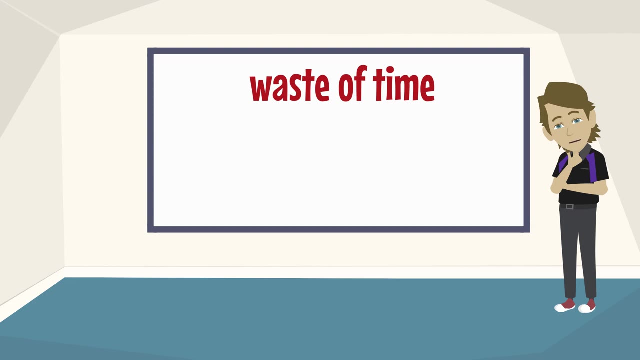 Could you make some time to show me how to use the new software? Yeah, sure, I'm a bit short of time. today, though, Our next expression is waste of time. Something that is a waste of time is a bad use of your time. 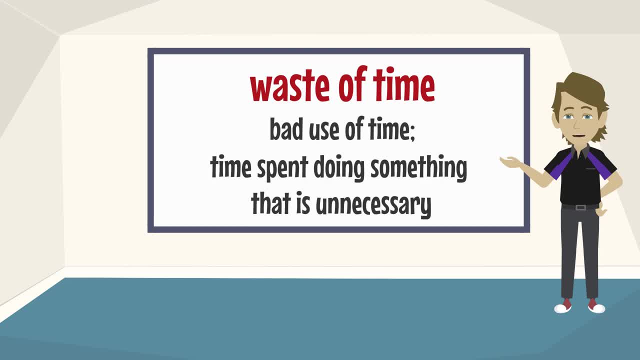 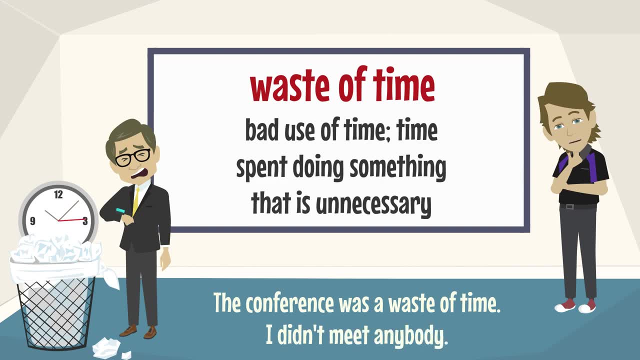 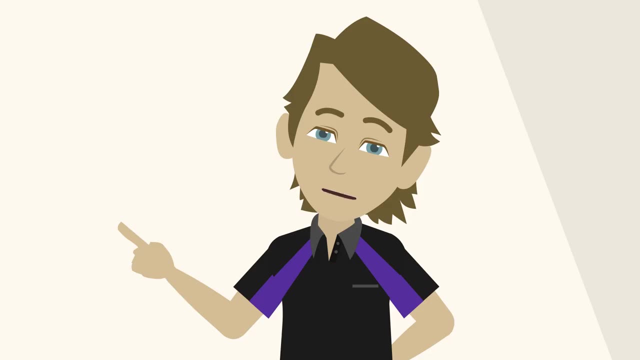 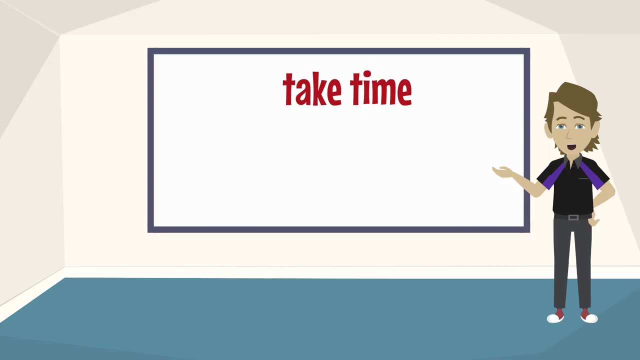 It's time spent doing something that is unnecessary. For example, the conference was a waste of time. I didn't meet anybody. Let's look at it again in context. I think the weekly report is a complete waste of time. Our next expression is: take time. 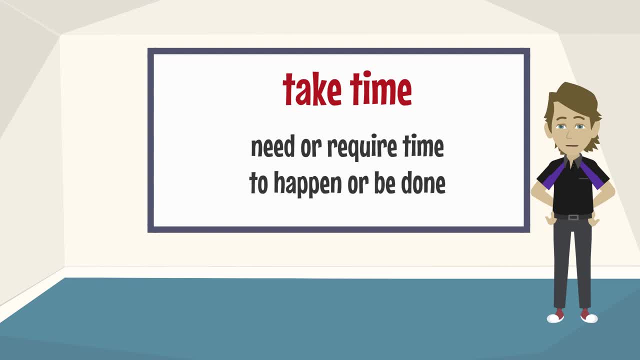 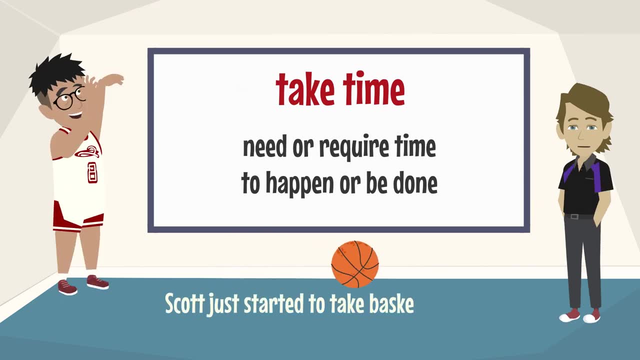 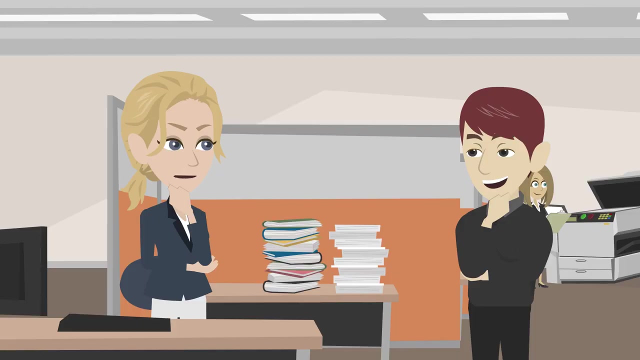 To take time is to need or require time to happen or be done. For example, Scott just started to take basketball lessons. It will take time. Let's look at it again in context. Sandy said it will take time for everyone to get used to it. 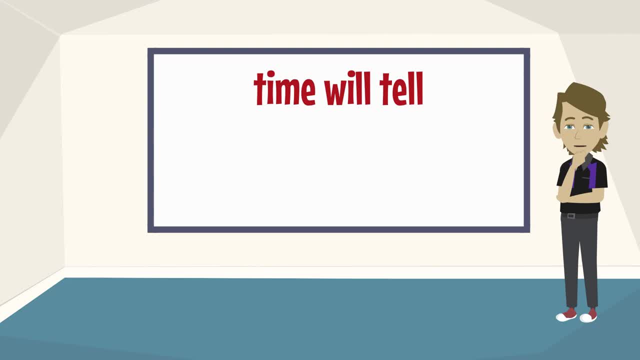 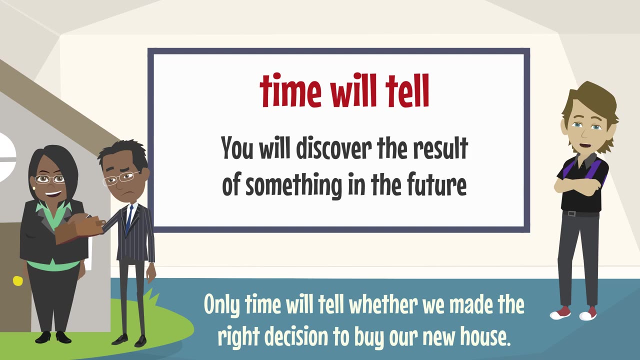 Our next expression is time will tell. We use the expression time will tell when we will discover the result of something in the future. For example, only time will tell whether we made the right decision or not. We made the right decision to buy our new house. 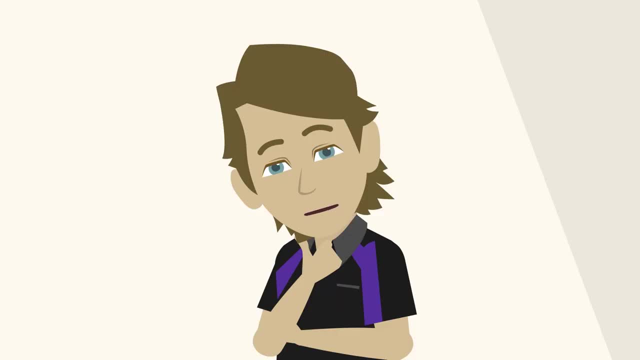 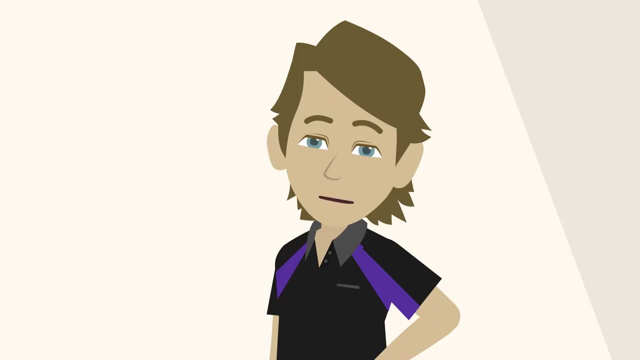 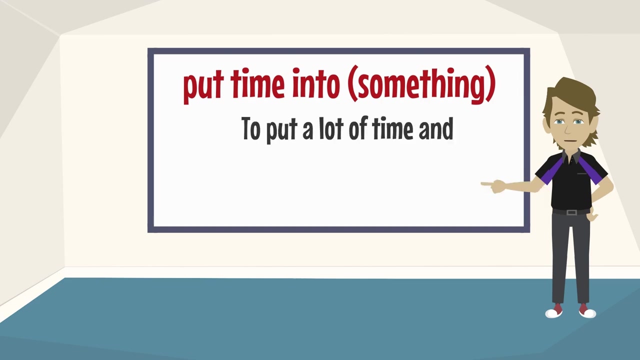 Let's look at this expression in context. again, Time will tell if it's a waste of time and money or not. And finally, we will look at three expressions. First, put time into something. This expression is used when we put a lot of time and energy into something. 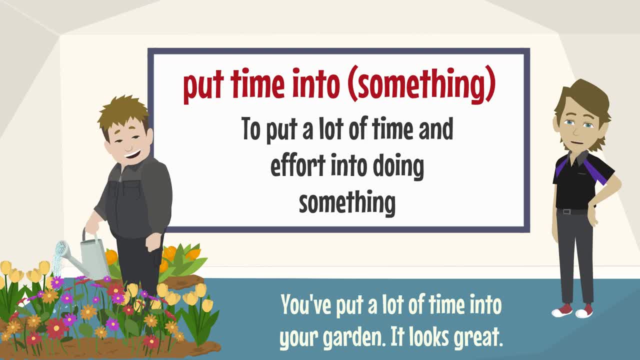 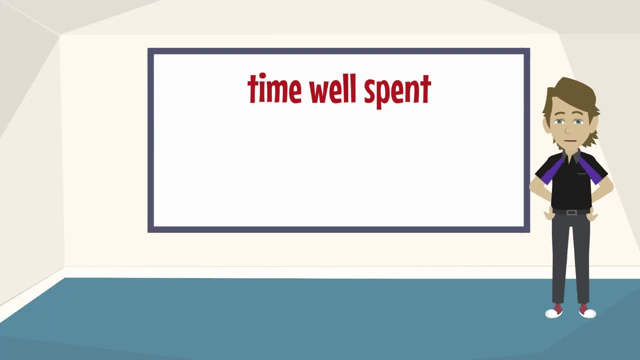 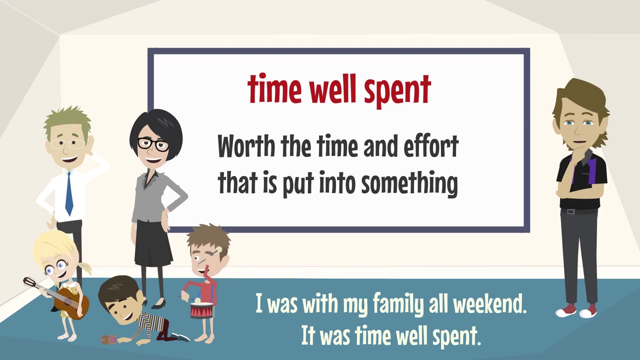 For example, you've put a lot of time into your garden. It looks great. The second expression is time well spent. We use this expression when something is worth the time and effort that we put into it. For example, I was with my family all weekend. 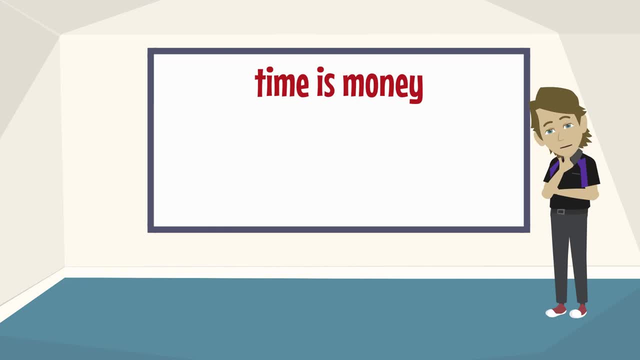 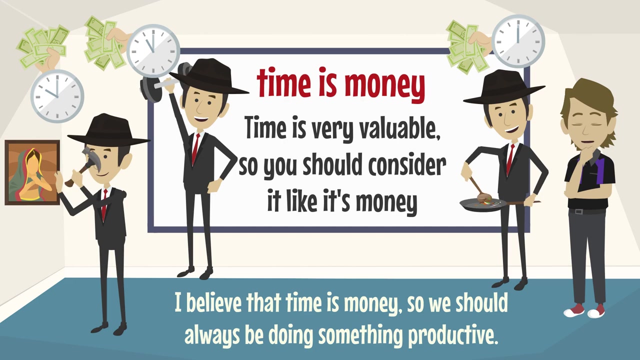 It was time well spent, And the final expression Is: time is money. This expression means that time is very valuable, So you should consider using time like it's money, For example. I believe that time is money, So we should always be doing something productive. 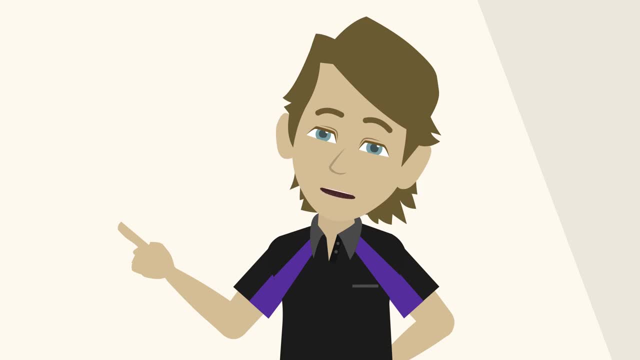 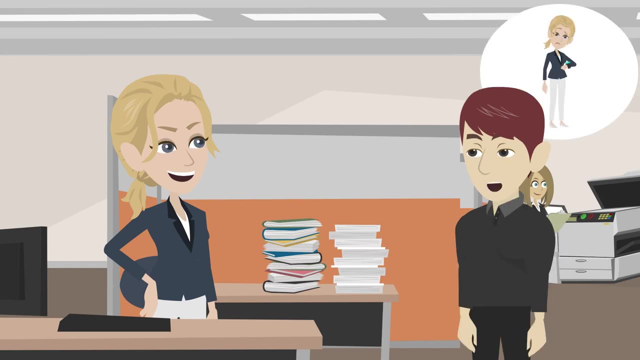 Let's look at these expressions in context again. It seems like you're putting a lot of time into it. It just doesn't seem like it's time well spent. Time is money, Dorothy. That's all for today's lesson. Thanks for watching. And see you next time.